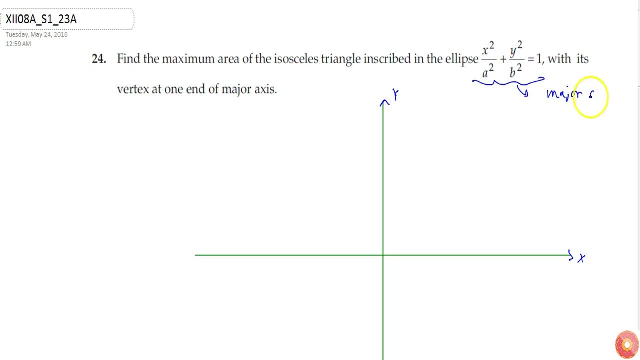 the ellipse has major axis on x axis, Then this will be something like this: So let's consider that the isosceles triangle inscribed in the ellipse has vertex at this major and one end of major axis. So this is nothing but a comma 0. Here, a minus a comma 0. Here. 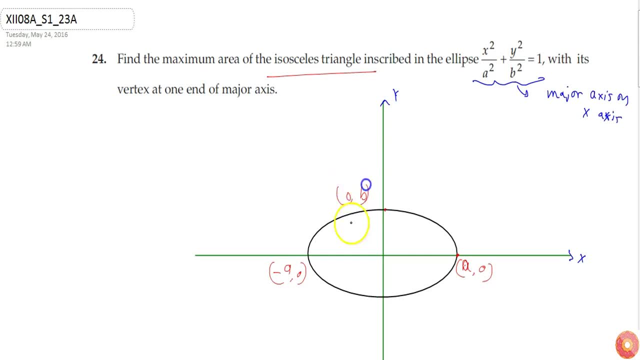 b comma, 0 comma b, and this is 0 comma minus b. So I know that two sides of isosceles triangle is equal. So I know that if two sides of isosceles triangle are equal, Let's say: 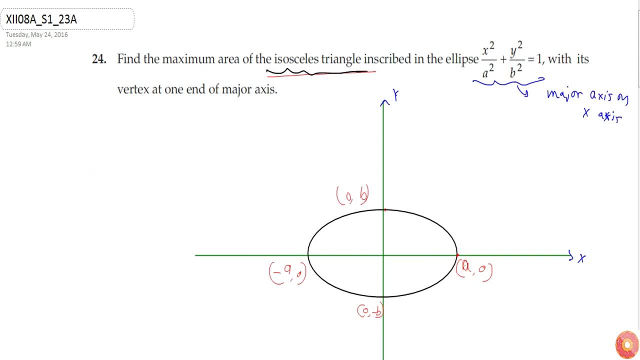 These are two of isosceles triangle and this is third side. so if these two sides are equal, then I can say that the X coordinate of other vertices will be equal. so I know that it's a standard coordinate, can be a standard point, can be written as, let's say, P a cos theta and B sine theta. this is a. 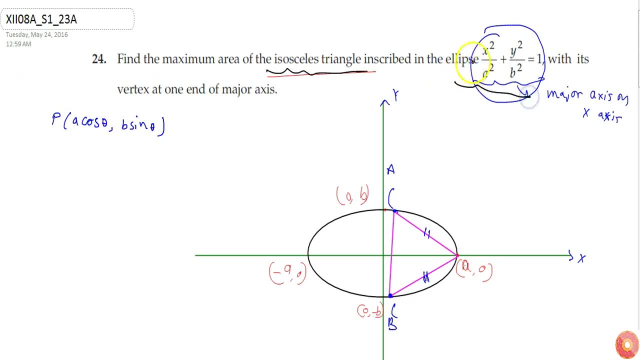 standard coordinate of ellipse, which area, which is you, which is equation, X square by a square plus Y square by B square is equal to 1. so if these two sides are equal, then the X coordinates of point A and point B will be equal, which will be a cos. 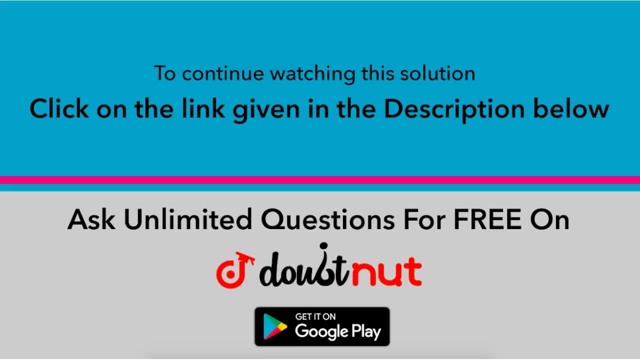 theta and a sine theta, a cos theta. watch the full video solution on the dot nut app.